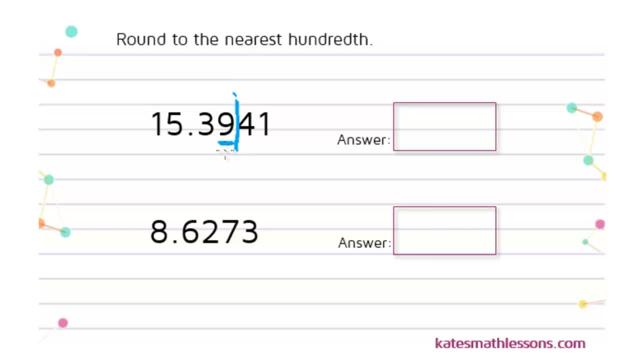 the number in the hundredth place stay the same or does it round up? In order to tell whether to keep it the same or to round it up, you look at the number after it. So we need to look at this four here And when you're telling whether to round or not, if the number 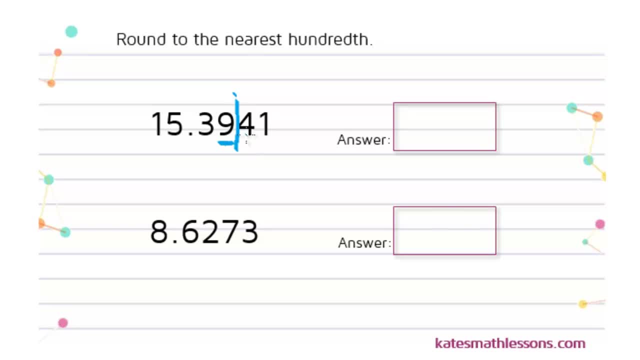 is five or greater, that means you need to round up. If it's four or less, that means you need to keep it the same. So since this is a four or less, that tells us that this nine just stays the same. So our rounded answer would be fifteen point three nine. 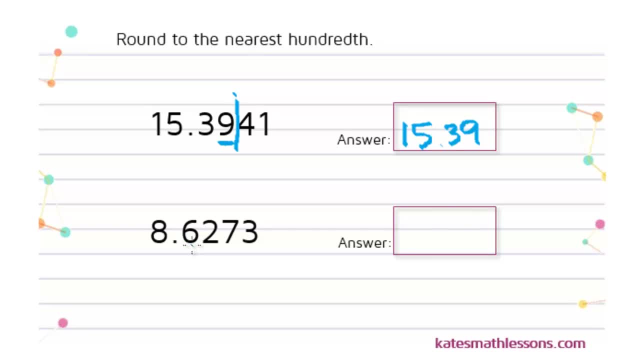 Let's do another one. The number after the decimal is the tenth place, so here the hundredth place is our two. so draw a line after the two. So the question we're asking is: does this stay a two, or do I round it up to a three In order to tell? I look at the number. 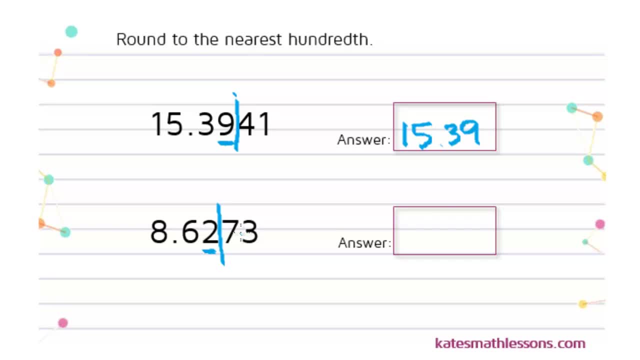 after it This number is five and a half. If it's five or greater, it's a seven. so that tells me that I need to round this two up to a three. So this rounded answer would be eight point six three. 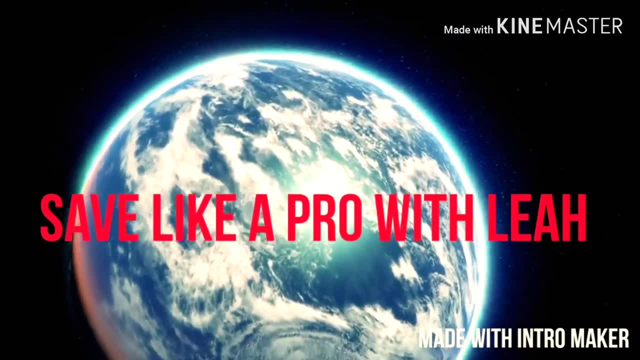 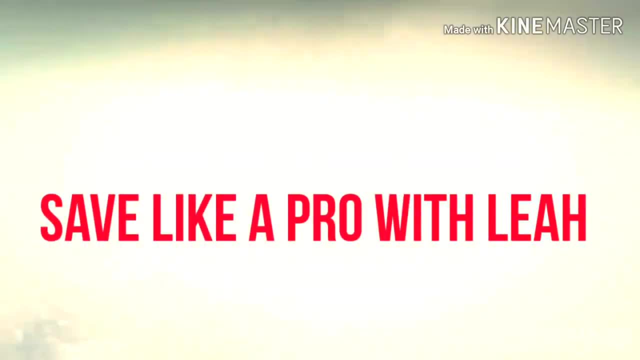 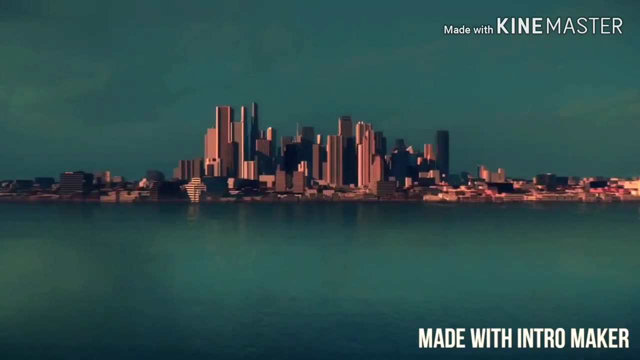 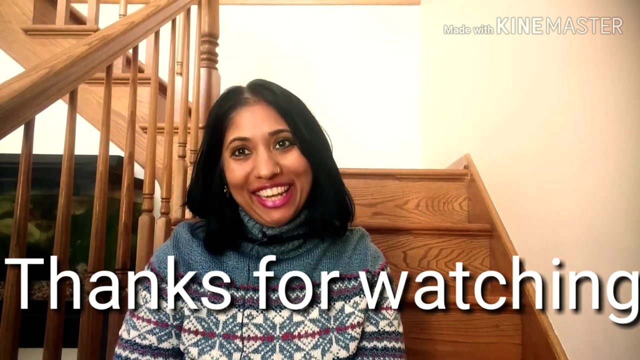 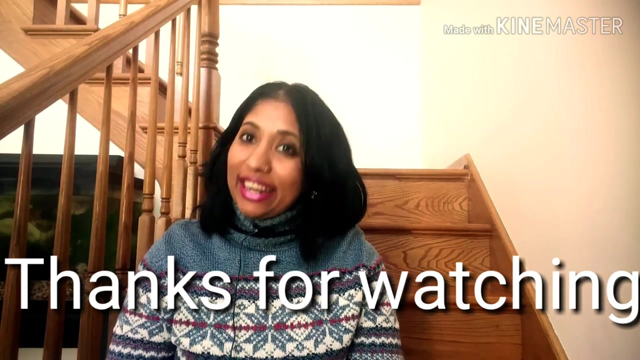 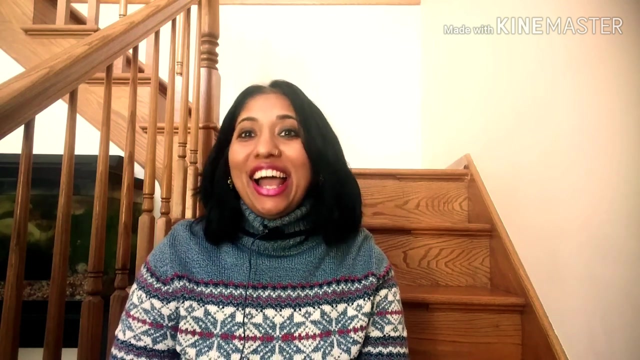 Hello everyone, welcome back to another episode of Save Like A Pro with Lea, one of my new subscribers. Welcome to my channel and I really appreciate that you are stopping by and if you are one of my faithful subscribers. I thank you so much for continuous support. Today I'm going to talk about 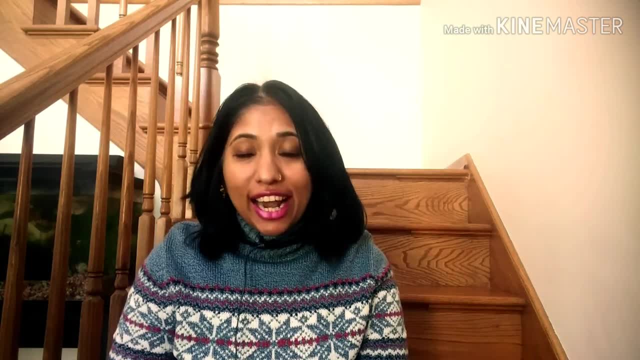 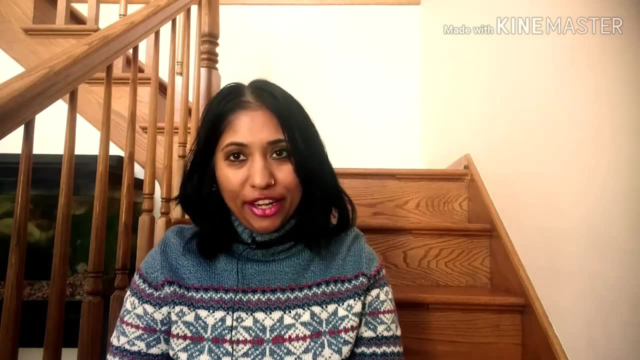 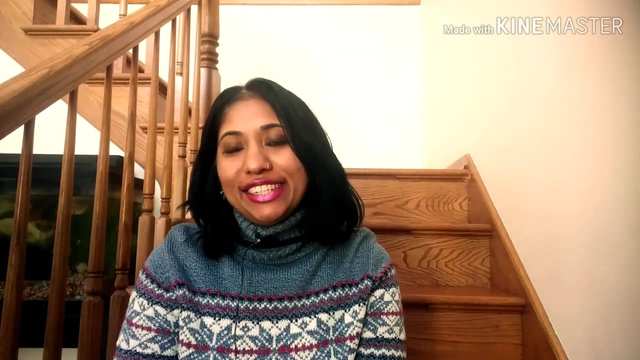 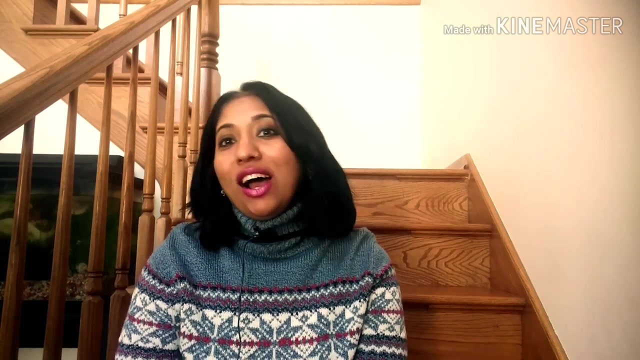 different cultures, eastern culture versus western culture- So you will know where I'm coming from and we are different than other people. I appreciate all type of cultures, ethnicity and diversity. I think diversity is one of the best thing any country can have, So we all can learn from different people. Yeah, today I'm going to talk about